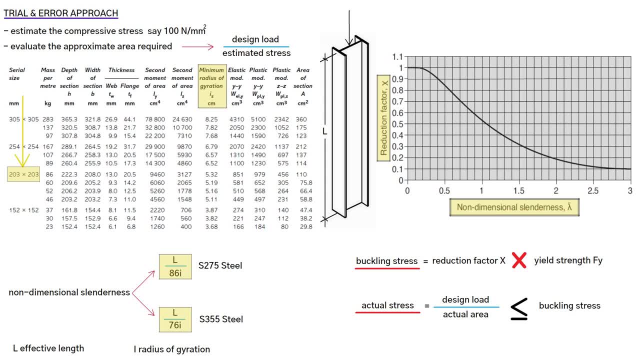 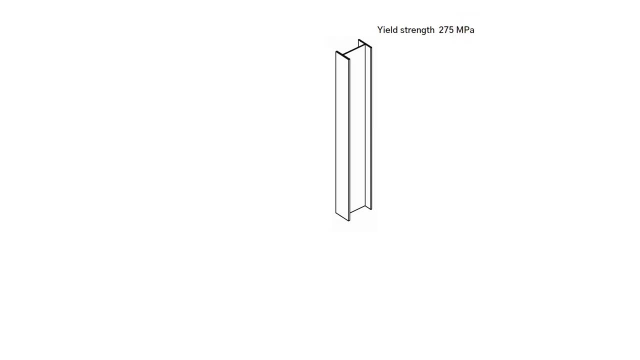 Therefore, we should select a bigger section. If it is substantially lower, then we should select a smaller section in order to improve economy. Let's start with the following application example: A pin-ended column with a yield strength of 275 newton per millimeter squared. 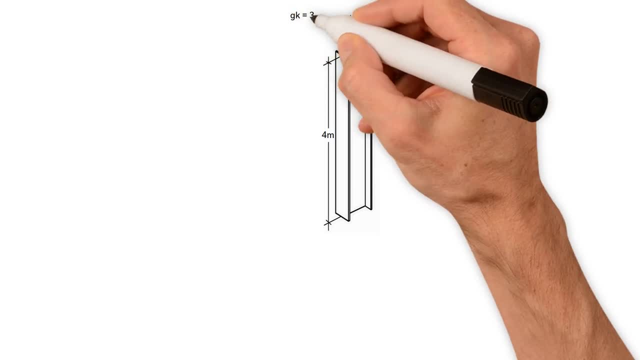 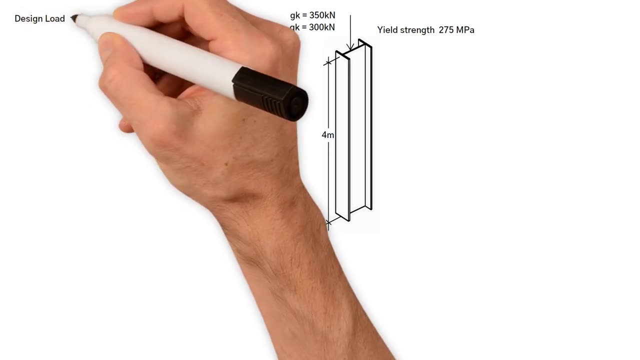 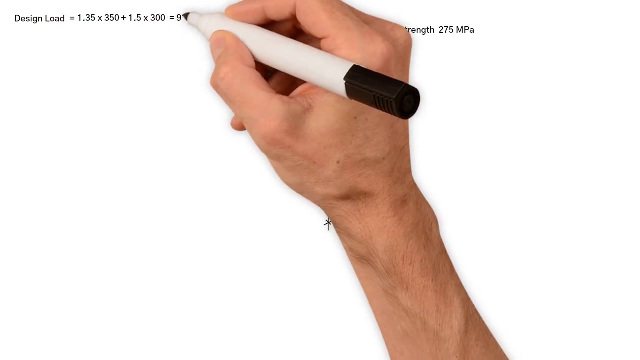 4 meter long, is subjected to axial permanent load of 350 kilonewtons and variable load of 300 kilonewtons. So the design load equals 1.35 times 350, plus 1.5 times 300, which equals 922.5. 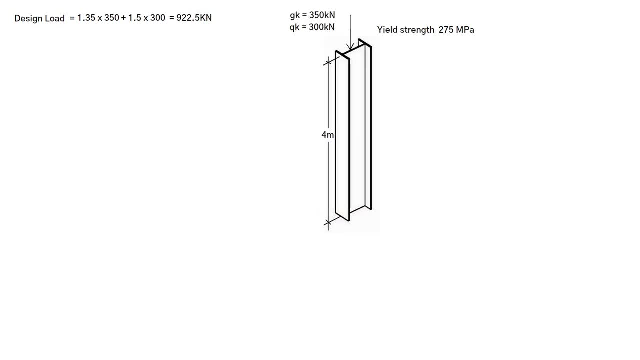 kilonewtons, As we mentioned earlier. the first thing we need to do is estimate the compressive stress in the column, Let's say 100 newton per millimeter squared, And evaluate the approximate area required. Hence, approximate area equals design load. 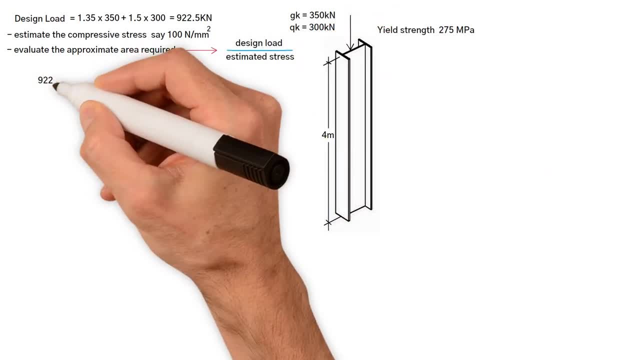 divided by estimated stress, which is 922.5 times 10 to 3 to convert to newton, divided by 100 newton per millimeter squared, and that gives us 9200 millimeters squared. We need to convert this to centimeter squared. To do this, we divide 9200 by 100,. 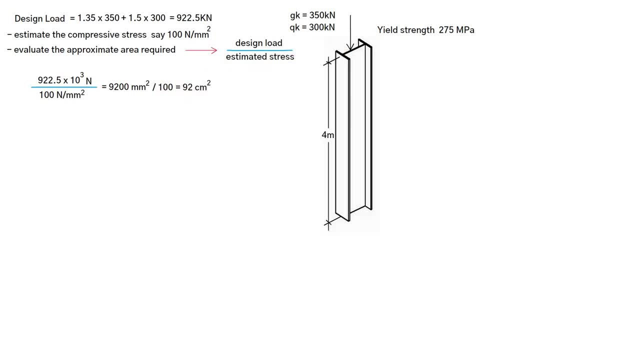 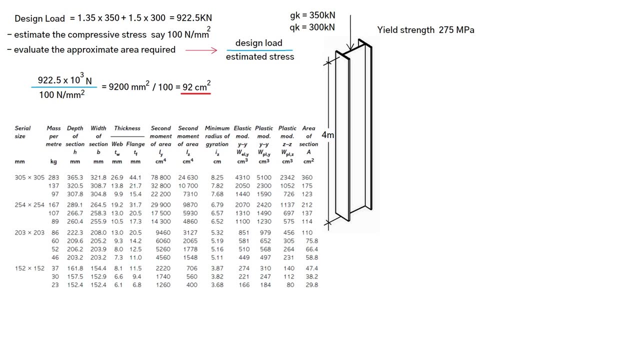 and this gives us 92 centimeters. Then we need to select a suitable column section size from the table and evaluate the non-dimensional slenderness. Let's try 254 by 254,. 89 kilogram per meter universal column which has the following properties: 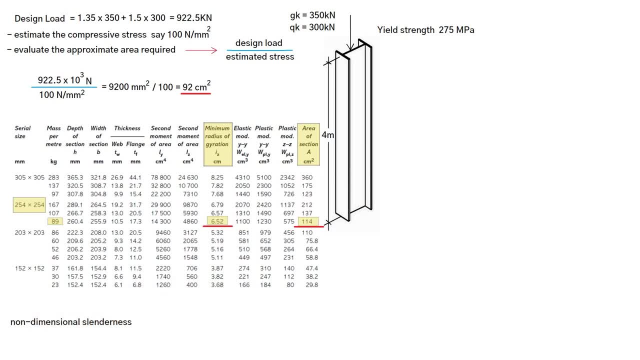 To evaluate the non-dimensional slenderness we need to use the following equation. Therefore, slenderness ratio equals 4000 millimeters divided by open bracket 80. Let's convert this to millimeter, So it would be 86 times 65.2.. 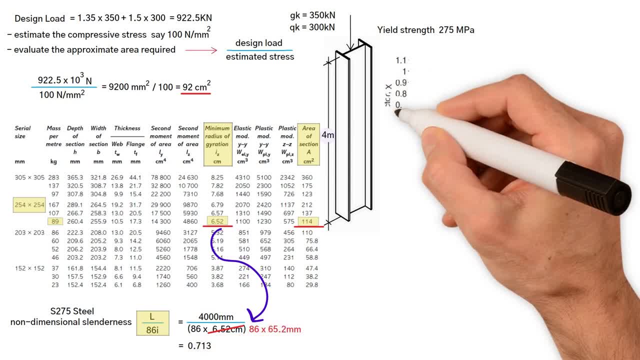 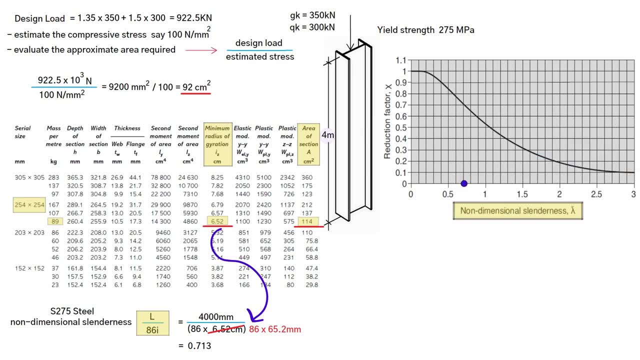 Our result is 0.713.. From the design curve we should be able to obtain the reduction factor, as we get a non-dimensional slenderness of 0.713.. If we extend the line to meet at this point with the curve, this gives us approximate figure of reduction factor. So if we extend the line to meet at this point with the curve, this gives us approximate figure of reduction factor, as we get a non-dimensional slenderness of 0.713..